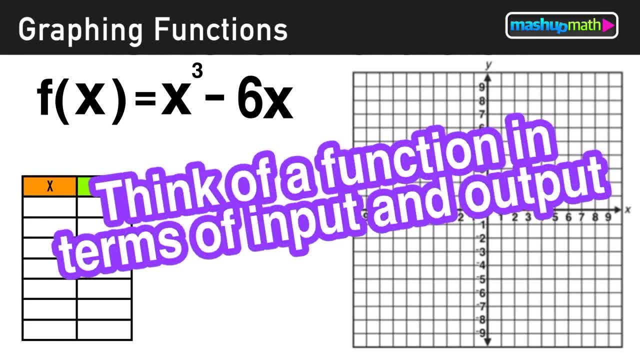 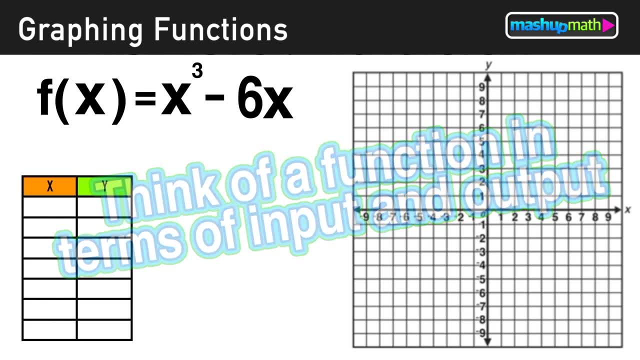 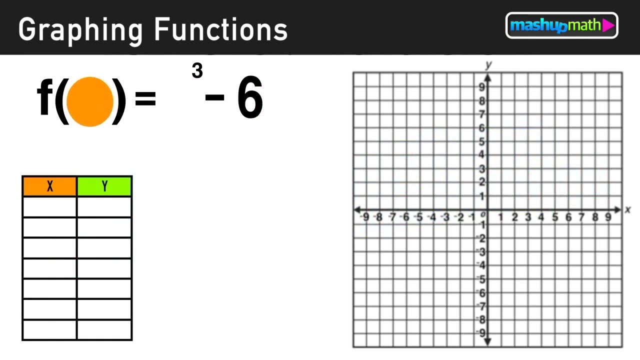 and output. That is, you input a value into the function and it outputs some other value. Now you probably already know that, by definition, x represents the input, But let's not think of it in terms of x. In fact, let's just get rid of the x's for now and think about inputting. 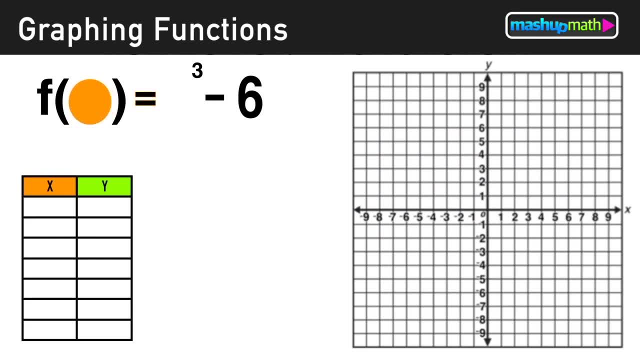 an orange circle. For this particular function I would have to take that input, that orange circle, and cube it first and then subtract 6x, whatever that orange circle is, from that. So again for this function, we take an input value, we cube it and then subtract 6x that. 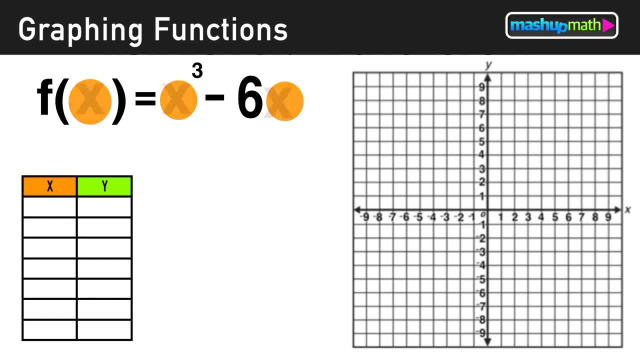 value from it and that result will be our output. So remember that x just represents whatever value we are inputting into the function And f of x just equals the output or the y value of the function. So for this function, what happens when we input zero? To find the output we have to. 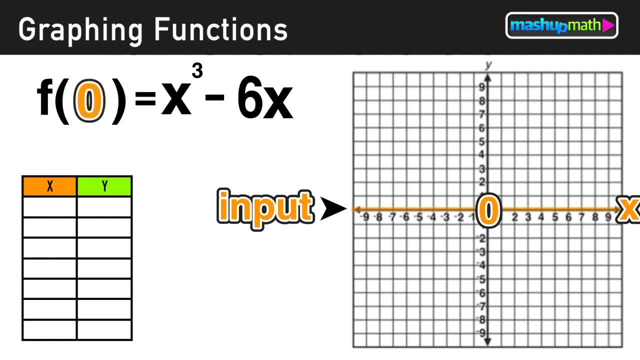 replace x in the original function with zero. So for every x in the function we replace it with a zero, and then we just evaluate. So in this case f of zero is equal to zero cubed, which is just zero Minus 6 times zero, which is just zero. and zero minus zero equals zero. 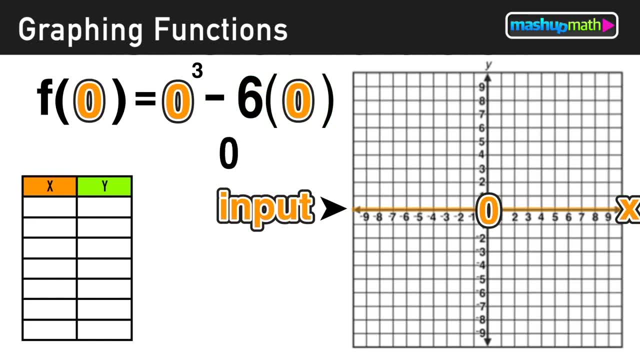 So for this function, when we input zero, our output is also zero and we have our first point that we can include on our table, and that point is zero, zero. So again, you input zero, you output zero and we know that this function is going to pass. 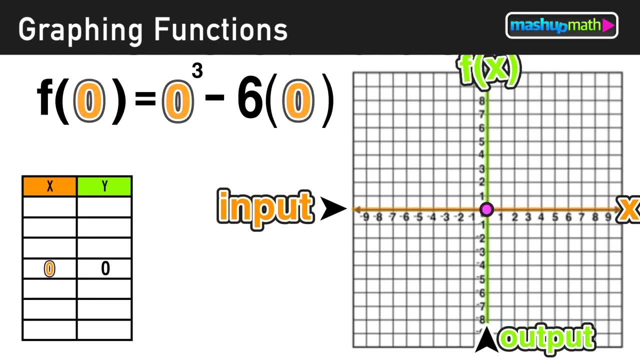 through the origin. So now what happens when we input one into this function? So when the x value is one, we replace x with one in the equation and then solve: One cubed is just one. Negative six times one is just negative six and one minus six equals negative five. 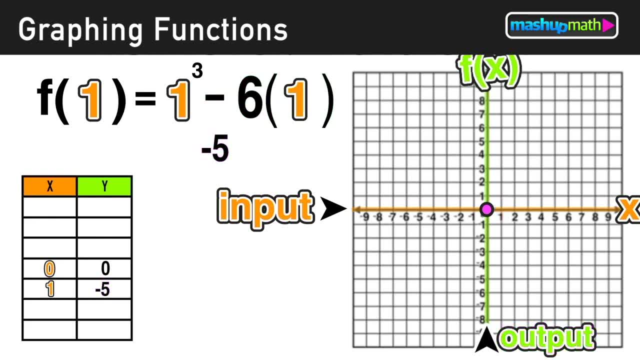 So now we can say when we input positive one, our output is negative five and that point one, negative five is another point that is on the graph of this function. We can continue this process for inputting a value of two. So when x is two in the original function, when we evaluate we get an output of negative. 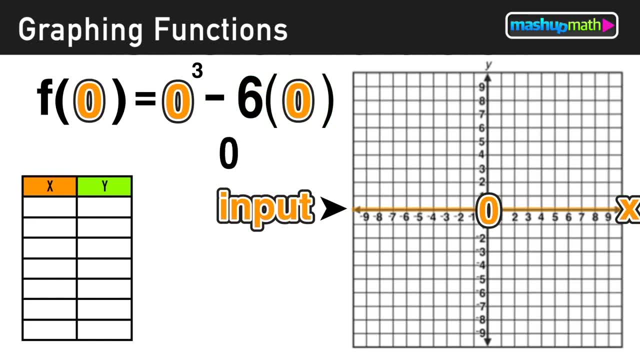 So for this function, when we input zero, our output is also zero and we have our first point that we can include on our table, and that point is zero, zero. So again, you input zero, you output zero and we know that this function is going to pass. 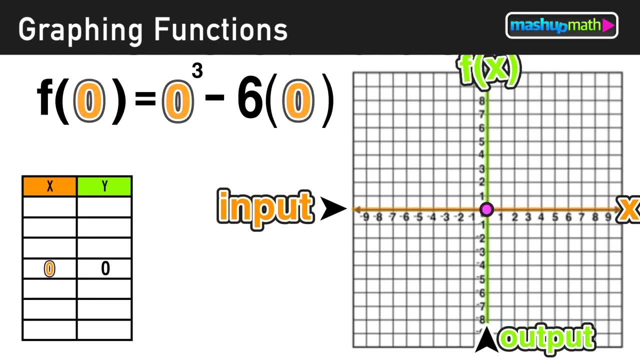 through the origin. So now what happens when we input one into this function? So when the x value is one, we replace x with one in the equation and then solve: One cubed is just one. Negative six times one is just negative six and one minus six equals negative five. 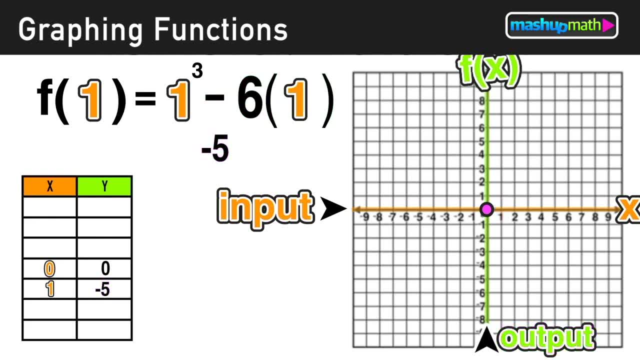 So now we can say when we input positive one, our output is negative five and that point one, negative five is another point that is on the graph of this function. We can continue this process for inputting a value of two. So when x is two in the original function, when we evaluate we get an output of negative. 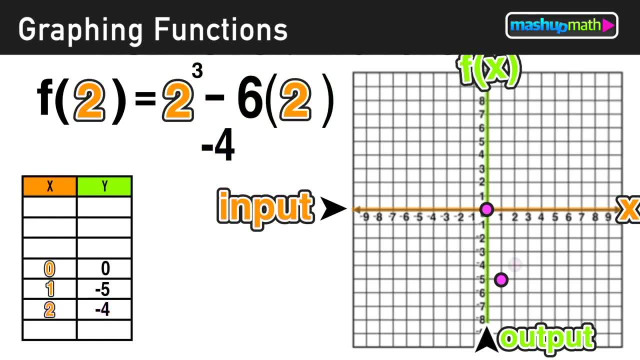 four, That's two cubed minus six times two And two negative. four is another point. that is on the graph of our function And when we input three we can see that three cubed minus six times three evaluates to nine. So when we input three, our output is nine. 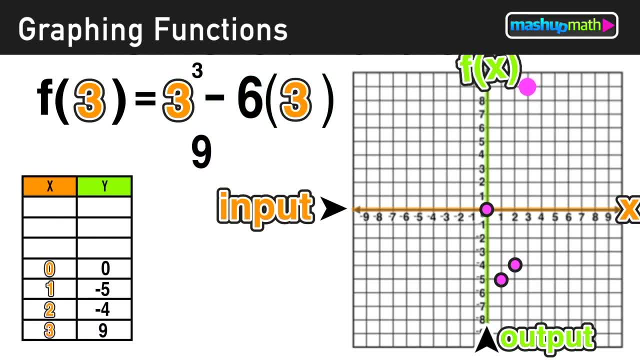 And the point three, nine, is yet another point, Another point on the graph of our function. And now we can continue this process of taking an x value, inputting it and then evaluating to get the y value of the output for the three additional negative values. 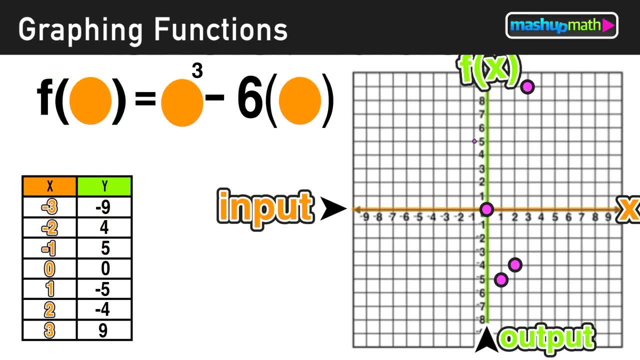 So once we find these outputs for each given input, we can graph the new points. One is at negative, one positive five, Another at negative, two, four And, the final point, at negative, three, negative nine. So now we can see that one is at negative, one positive five. 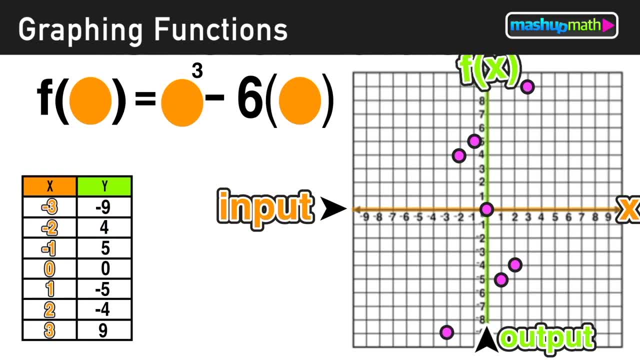 And the final point, at negative three, negative nine. Now we have a whole bunch of points here, okay, on our graph that represent our function. Now we have to be careful when we connect these points to draw a curve that correctly reflects this function. So to do that, we want to move from left to right as we connect the points. 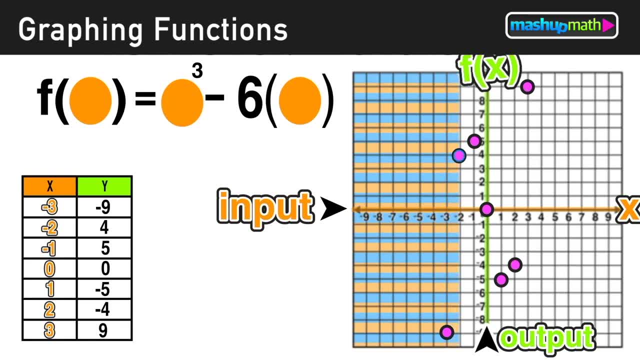 So we will start with the first point that is furthest to the left And then move to the next furthest to the left point And connect those with a curve And continue this process. Okay, Notice that your line is curved and not totally straight and rigid as you move from point. 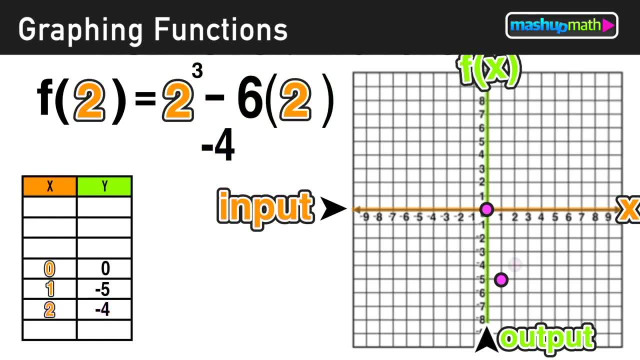 four, That's two cubed minus six times two And two negative. four is another point. that is on the graph of our function And when we input three we can see that three cubed minus six times three evaluates to nine. So when we input three, our output is nine. 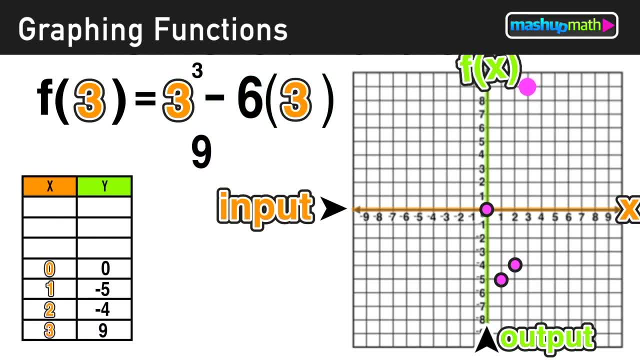 And the point three, nine, is yet another point, Another point on the graph of our function. And now we can continue this process of taking an x value, inputting it and then evaluating to get the y value of the output for the three additional negative values. 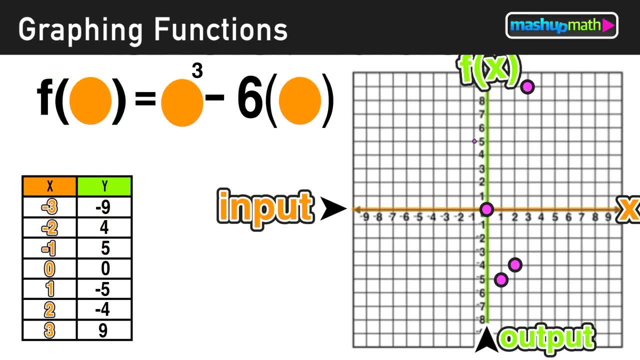 So once we find these outputs for each given input, we can graph the new points. One is at negative, one positive five, Another at negative, two, four And, the final point, at negative, three, negative nine. So now we can see that one is at negative, one positive five. 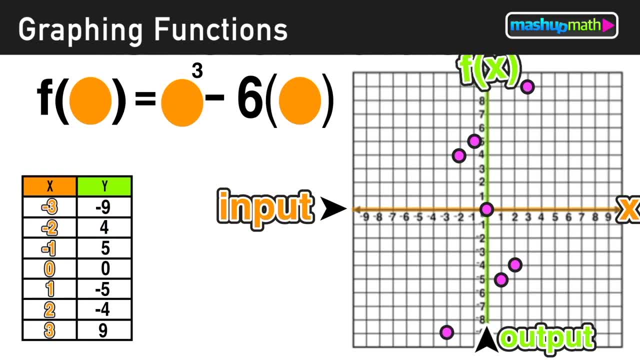 And the final point, at negative three, negative nine. Now we have a whole bunch of points here, okay, on our graph that represent our function. Now we have to be careful when we connect these points to draw a curve that correctly reflects this function. So to do that, we want to move from left to right as we connect the points. 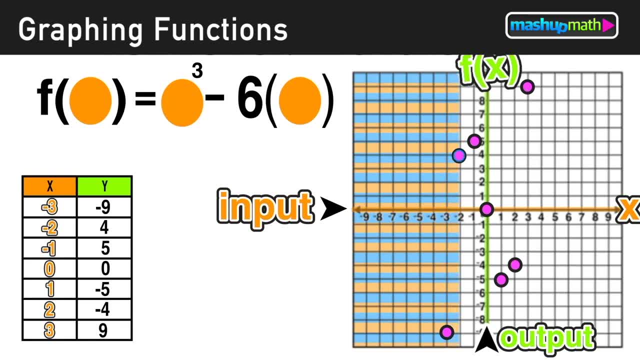 So we will start with the first point that is furthest to the left And then move to the next furthest to the left point And connect those with a curve And continue this process. Okay, Notice that your line is curved and not totally straight and rigid as you move from point. 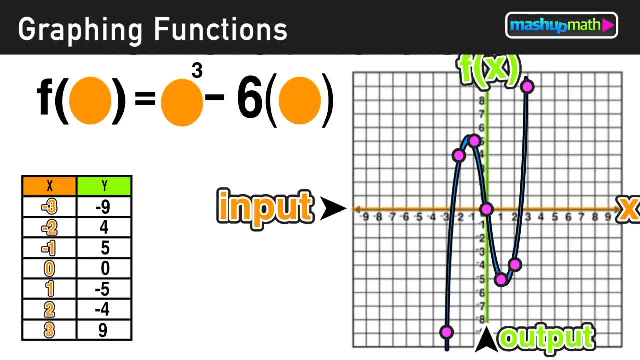 to point And we can continue this process to complete the graph of the function. And if you are familiar with cubic functions, this image should make sense, since we know that a cubic function has that peak and valley kind of curve shape to it. And on the last note, just remember that this process can be used for graphing any function. 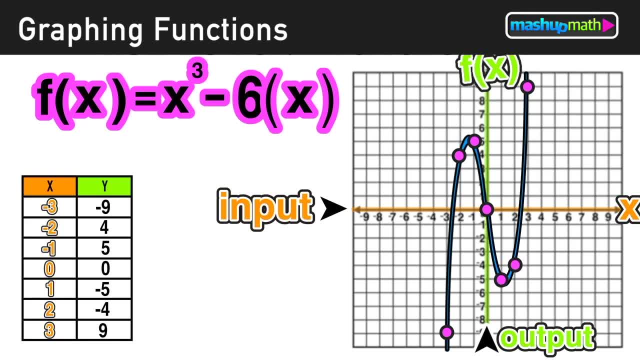 And that's what we're going to be doing today, And that is, you take input values, You put them into the function and evaluate And the result is your output, And you use those x and y values to find the points that are on the function which you 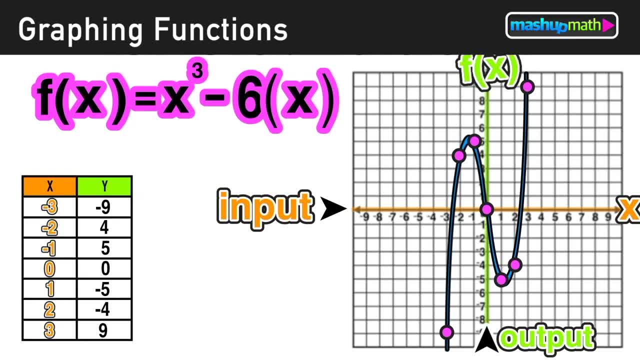 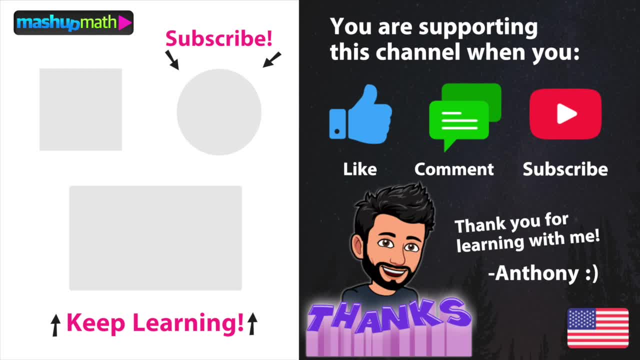 can plot and eventually construct a graph, And that's really all there is to it. So thanks again, guys, for stopping by, and we'll catch you guys next time. Bye, Bye, Bye.